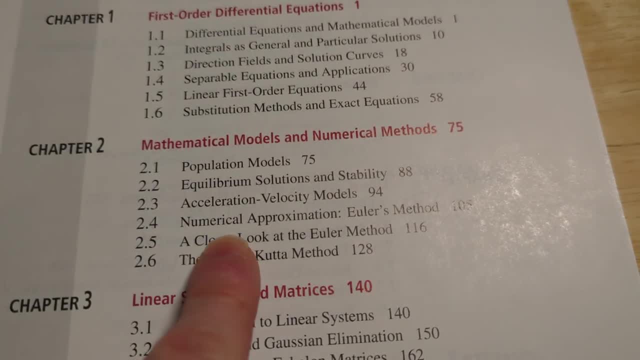 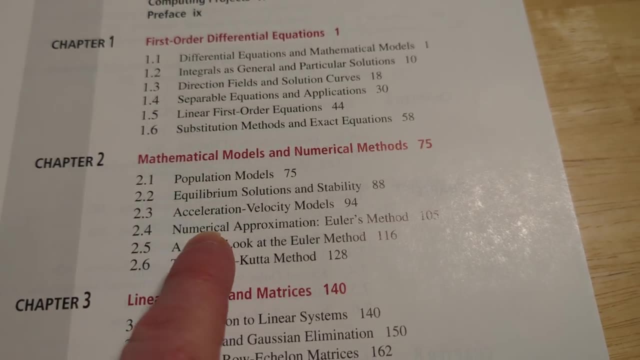 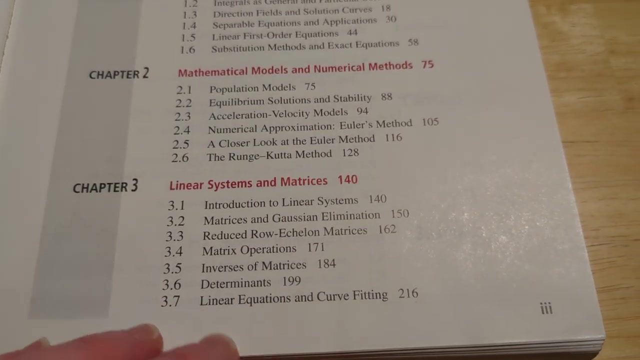 methods, And then here you have some stuff at the beginning as well. Chapter two is on some applications and some numerical methods. So we've got some models and then some more models and then some numerical methods here. Three is on linear systems and matrices. So this is something. 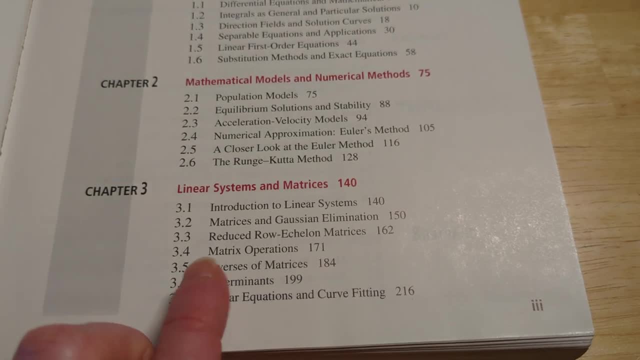 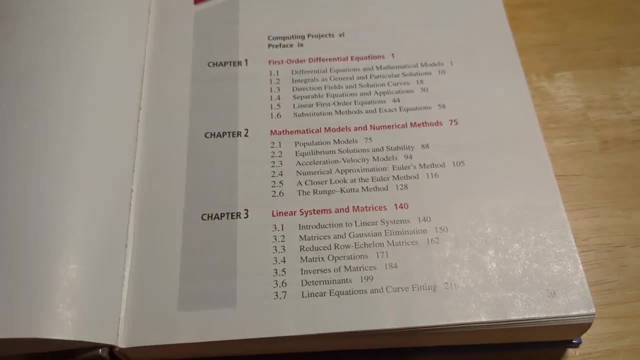 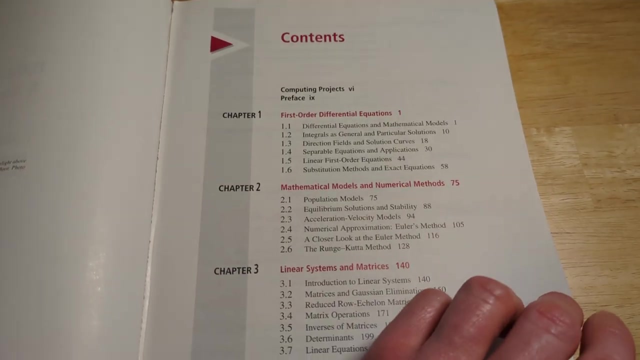 that you probably wouldn't see in another differential equations book. So very unique in that regard already in chapter three, something you're not going to get in other math books. By the way, the prereq for this, I would say, is a calc two course. You want to know how to integrate fairly well before tackling. 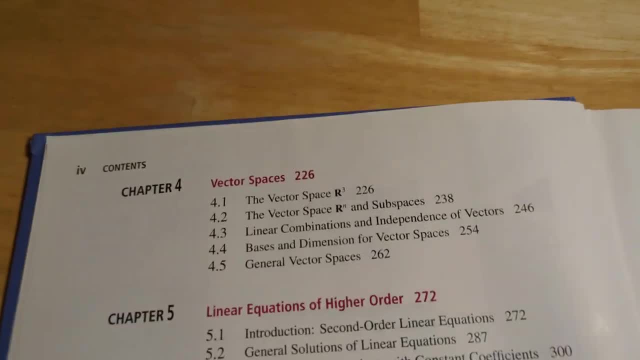 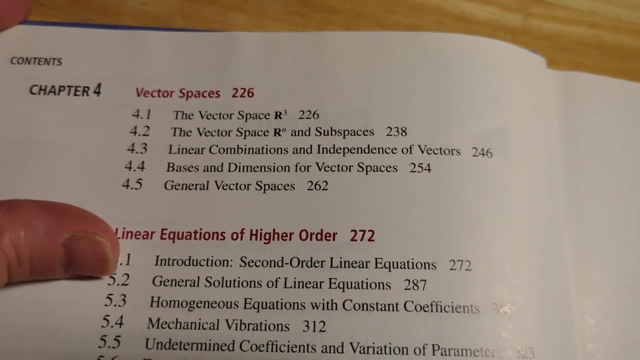 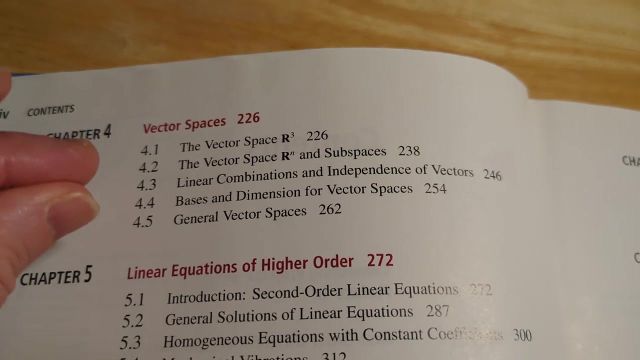 differential equations And look at this, This is awesome. Vector spaces, right, The vector space R3, the vector space Rn and subspaces. So again, not something that you typically get in an introductory differential equations book. A lot of DE books don't talk about vector spaces. 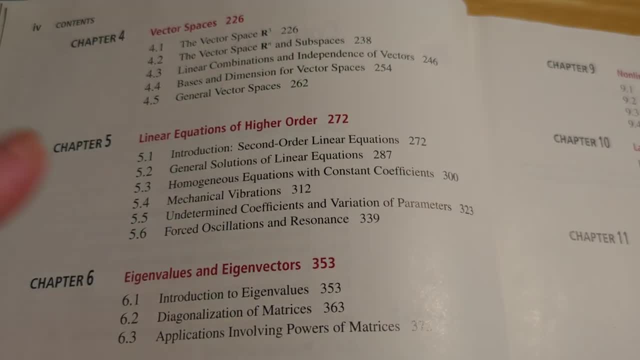 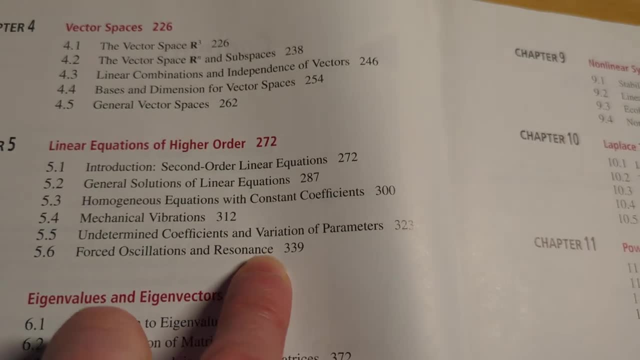 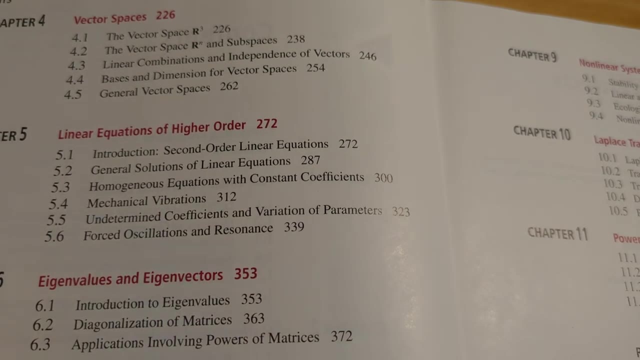 That's what this is. here There's forced oscillations and the resonance. You also have some other techniques like variation of parameters and some more applications here in the section on mechanical vibrations. Chapter six is on eigenvalues and eigenvectors- Again, very 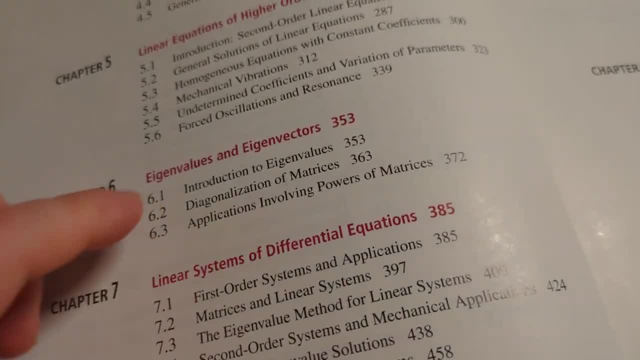 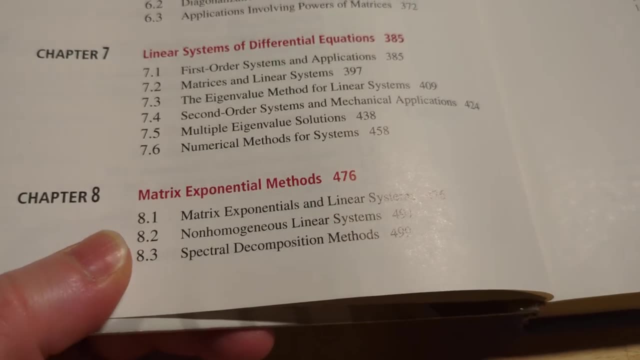 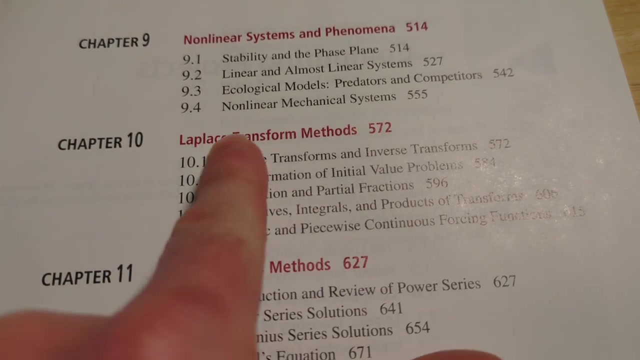 unique in that regard. Most introductory differential equations books don't cover this. Linear systems- really nice topic. Matrix exponential methods- Again something you typically don't see in a DE book, Laplace transform methods. This is something you usually see. However, I want to emphasize that there are 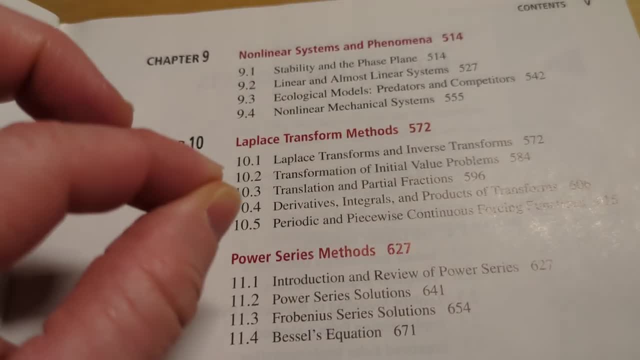 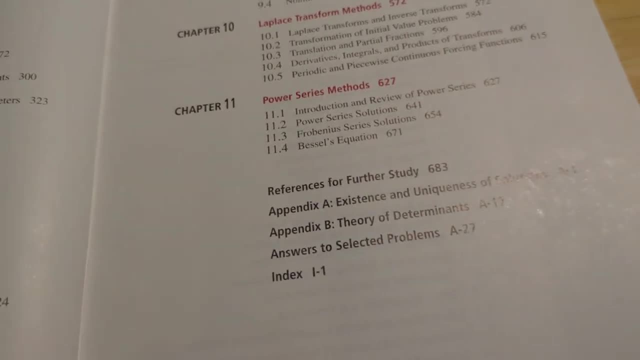 certain things in some of these sections, like little subtopics that you typically don't find in other books: Power series, methods. This is something that is found in most books, And then you have answers to some of the problems. I would say that this is a fairly deep 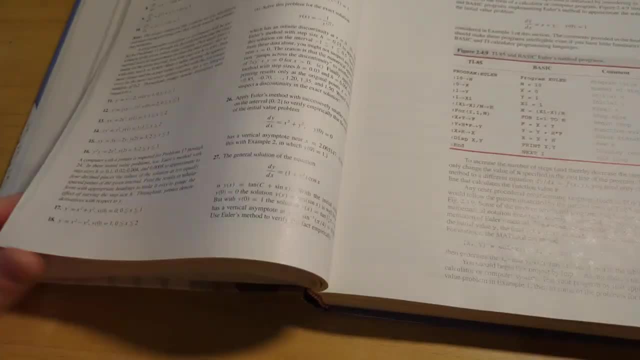 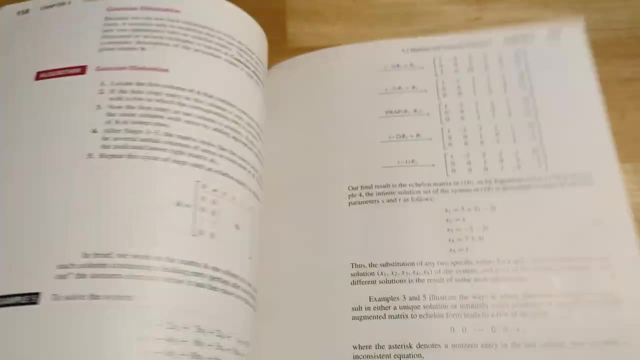 fairly decent book. It reads fairly well. I mean, it's a math book, It's a differential equations book, So it's going to take you some effort to work through, But I definitely recommend it And I will leave a link in the description in case you want to check. 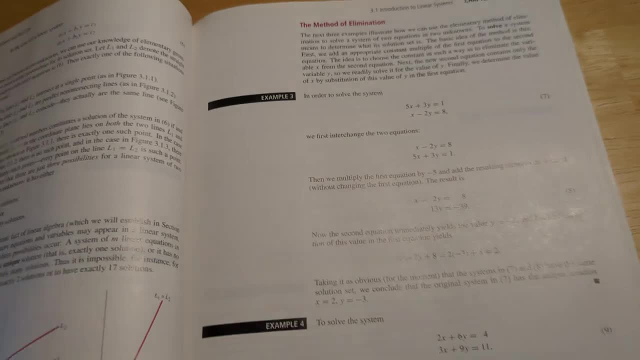 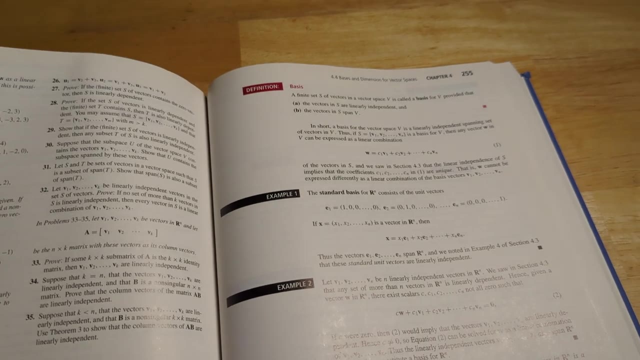 it out And I'm sorry, I just got to give it a whiff here. Oh, it smells so good, Smells so good. I've had this book for, I want to say, over 10 years now, And it's a good book. 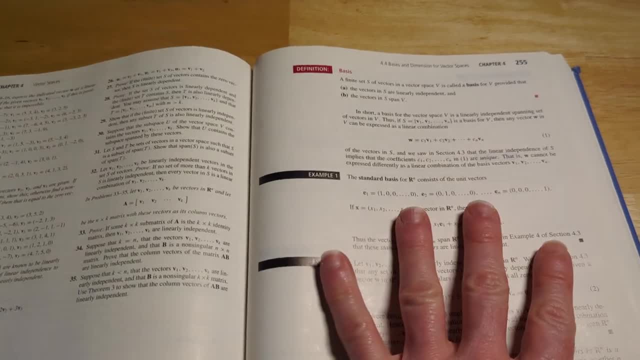 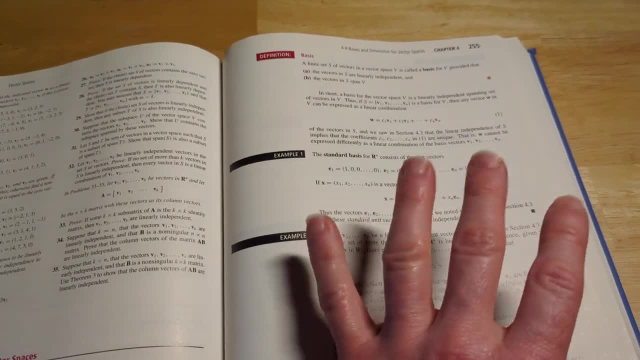 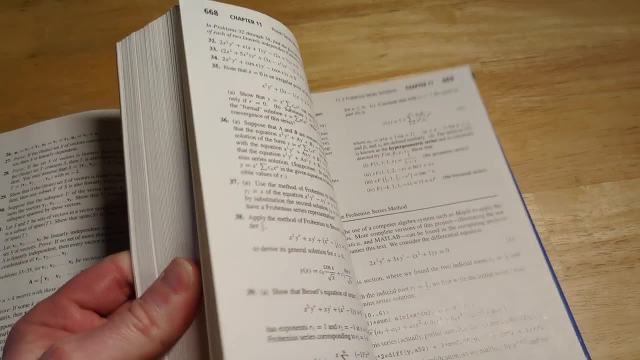 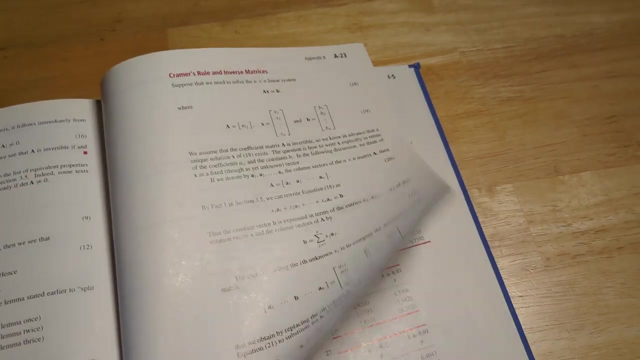 book has interesting examples, interesting problems and, again, topics that you don't typically find in other books. As far as the answers in the back of the book, you do have some answers. Let's take a look at those now. Let's see what we get here. So these are answers. 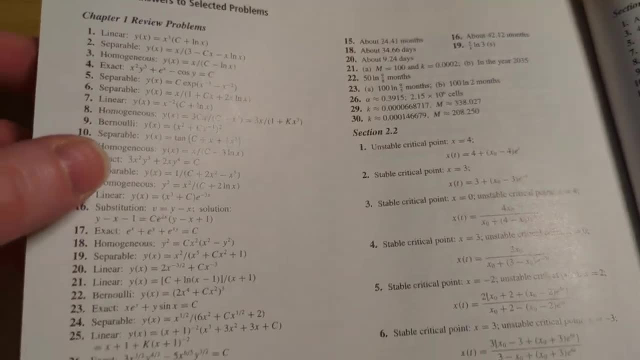 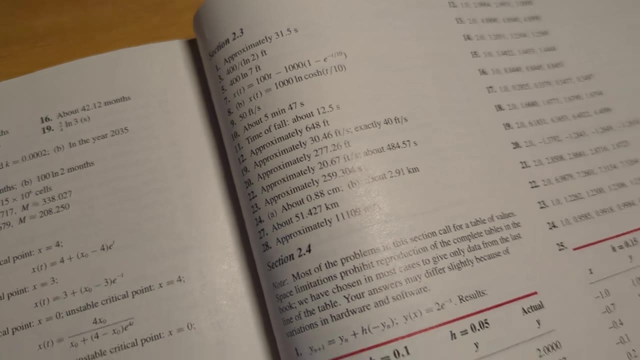 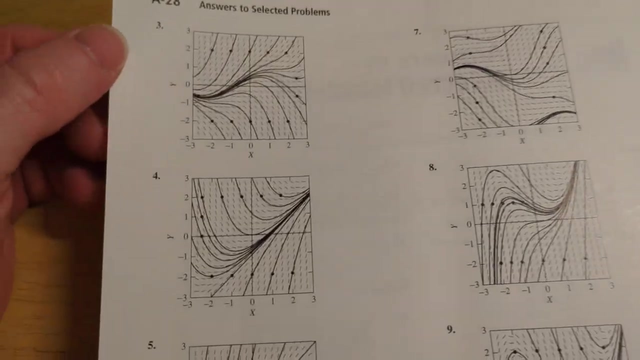 to review problems. Looks like you get all of those, Okay. and then here you see some of the answers in the back of the book. Now, you don't get all of the answers, but you do get a lot of answers. This is selected problems and you notice here. 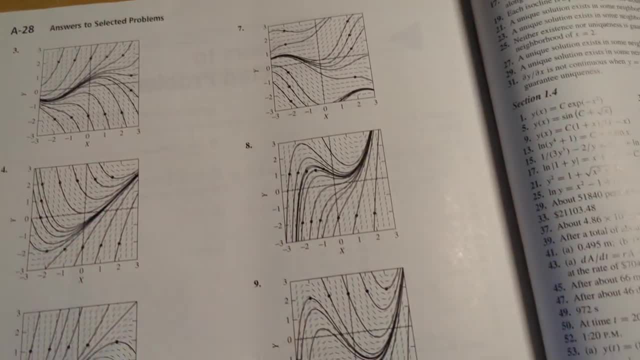 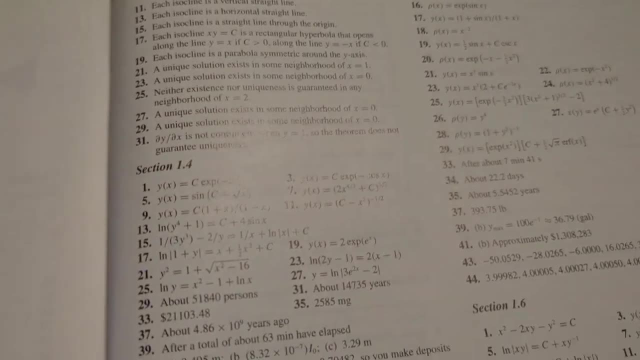 it's like three, four, five, six, seven, So it looks like it's giving you all of them, but it doesn't quite give you all of them. For example, here you see it's missing the even ones, but sometimes they give you more, Like for example, here's: 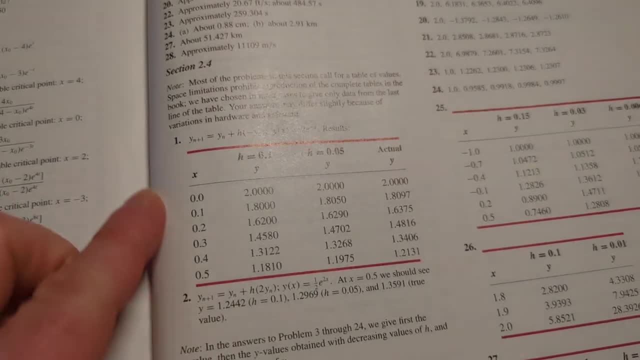 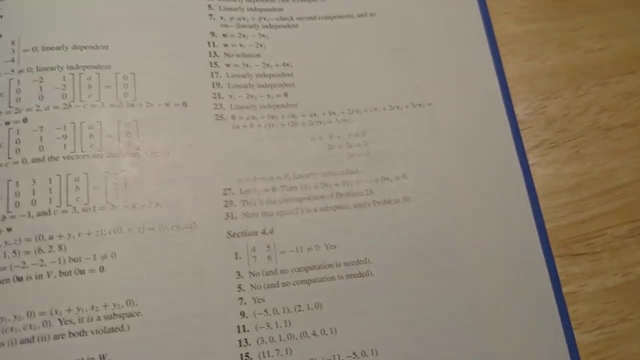 2.4 and you've gotten 1,, 2,, 3,, 4,, 5,, 6,, 7,, 8,, 9,, 10, etc. So pretty random. You've got some answers in the back of the book and it looks like it's more than the odds. 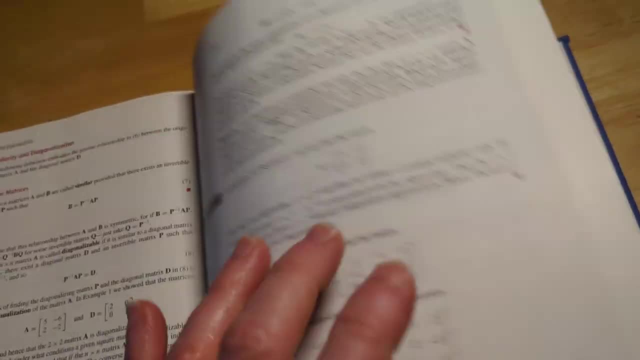 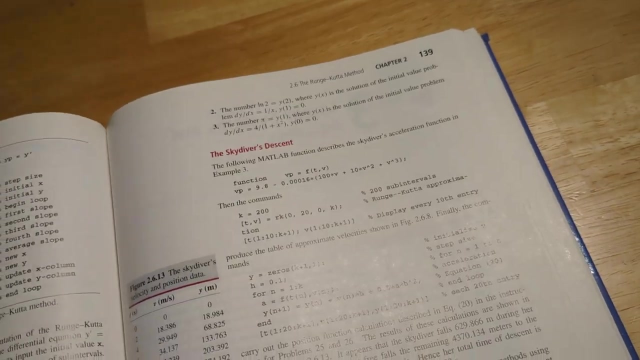 because you do get some even ones as well. The exercise selection in each section is pretty good. I would say it's fairly standard. Let's jump to like a common section that we would see in most books. Let's go to the beginning, so you. 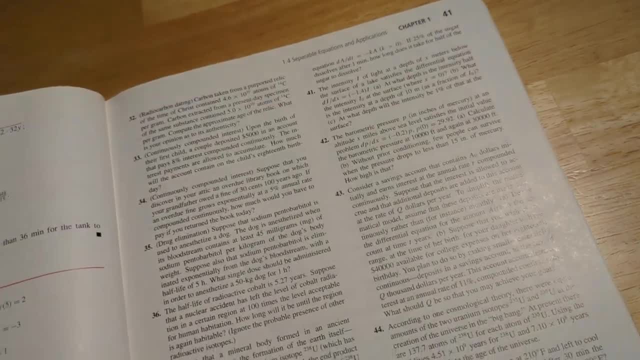 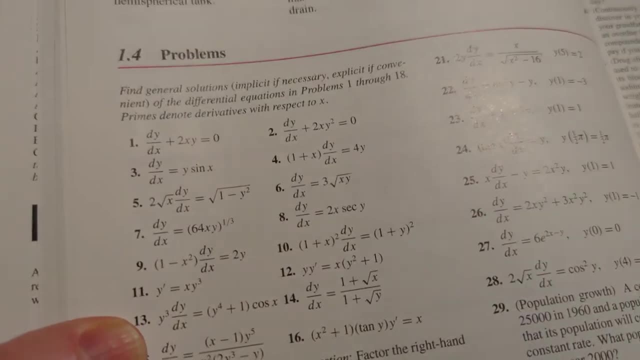 can see something that you don't know. Let's see what you would learn at the beginning of the course. For example, here's one. 1.4 is on separable equations and applications. This is something you can learn right away, Like if you bought this book you could start. 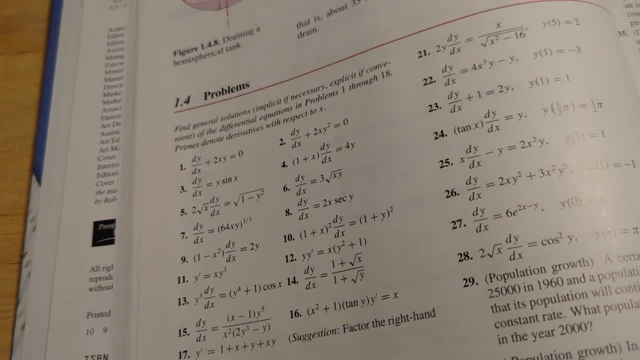 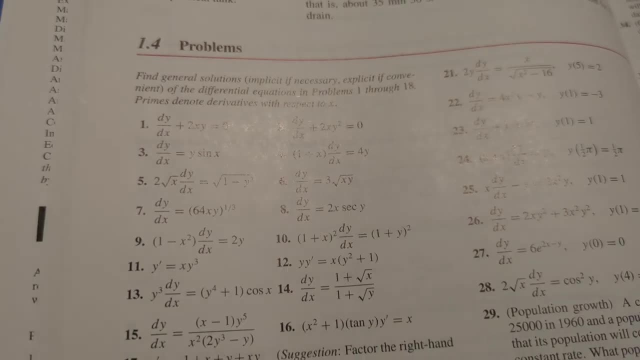 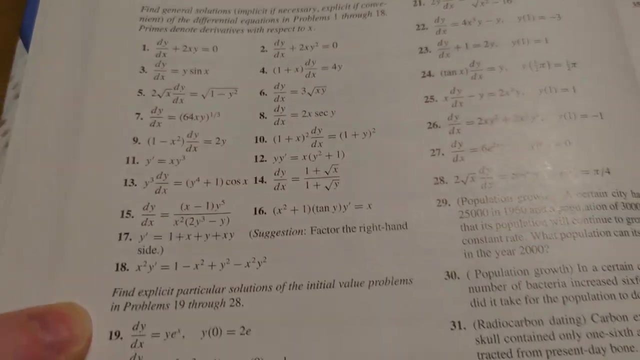 with this section. You can start in section 1.4.. You can skip everything else and start here and start solving differential equations. So these problems seem to be pretty easy, but they do get harder. So you get a lot of selection here in terms of exercises And here you have some initial value problems that 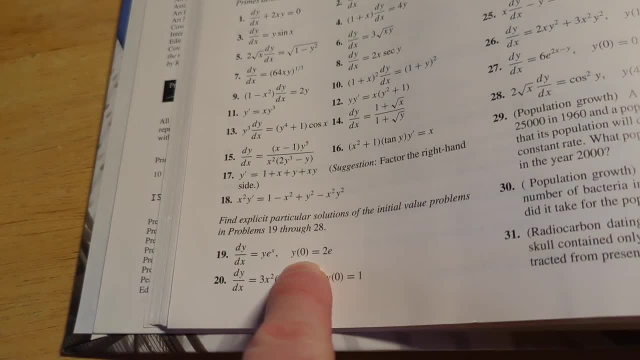 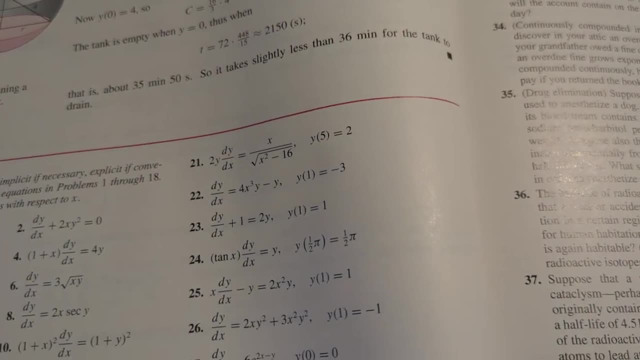 basically means you have the differential equation, and this here is called an initial condition, And you use this to find your constant at the end of the problem. So you've got a bunch of those there, And then you've got some applications here. These are pretty easy as well, Even though they're word. 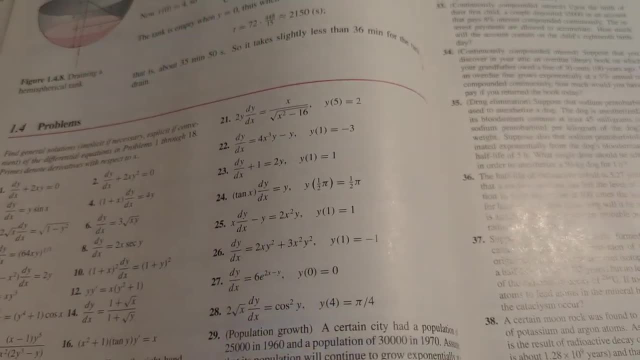 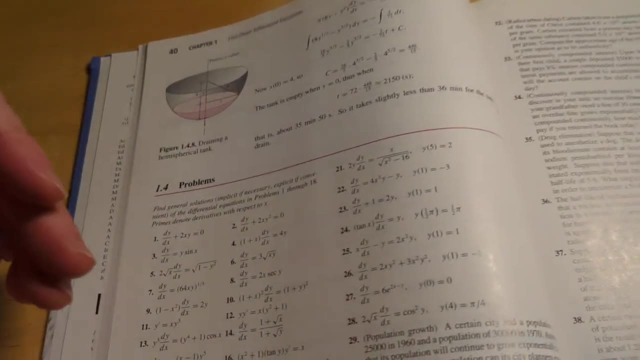 problems. they're not that hard. So I would say it's a good selection, A nice, nice selection of problems. And again, it's good practice. if you're taking a DE course and you want extra practice problems, What you can do is you can go. 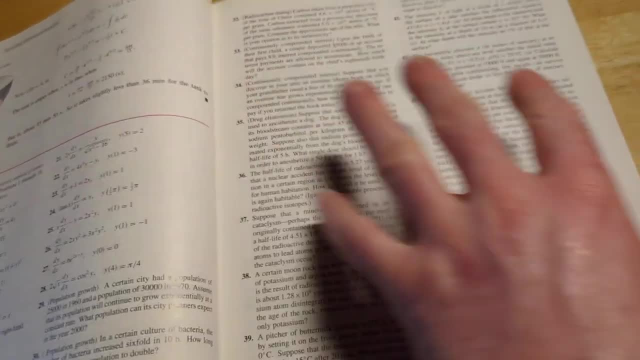 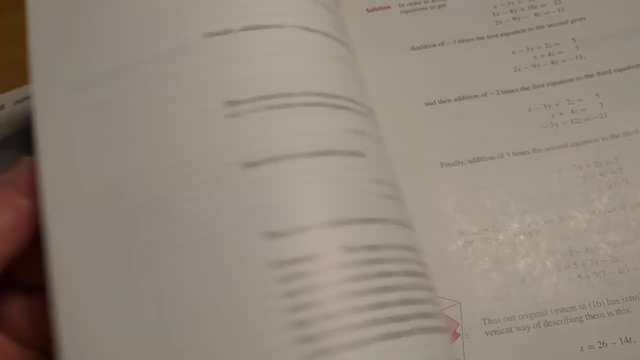 through a book like this and then you can just do the odd ones and then you can check your answer in the back of the book. But kind of a cool book if you want to learn some DE or if you want to learn linear algebra, It's certainly a very 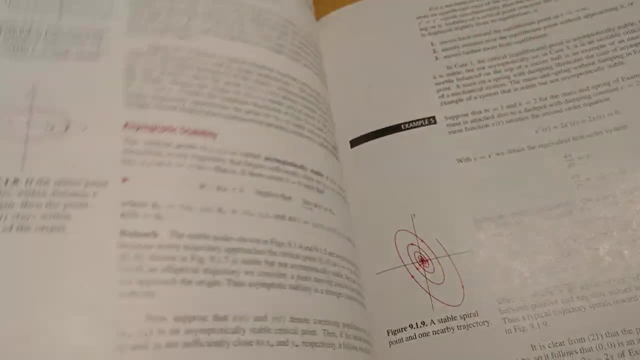 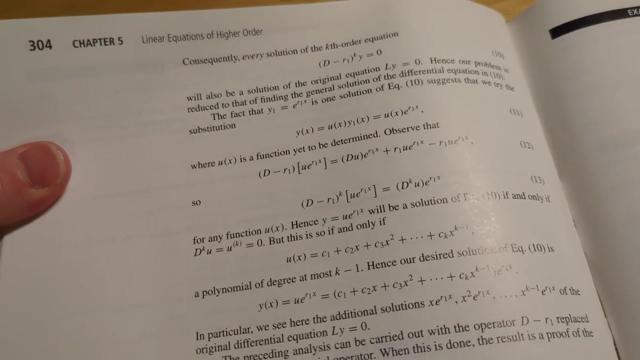 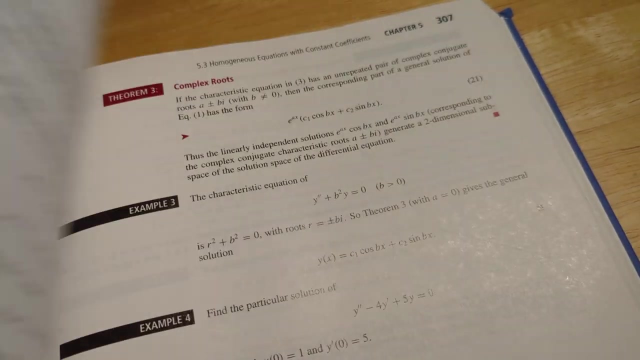 gentle approach to linear algebra. Again, I would say the prereq for something like this is calc 2.. This is the section on higher order DEs. Yeah, pretty cool, homogeneous equations with constant coordinates. Let's look at the exercises here. Let's jump to those. These are really 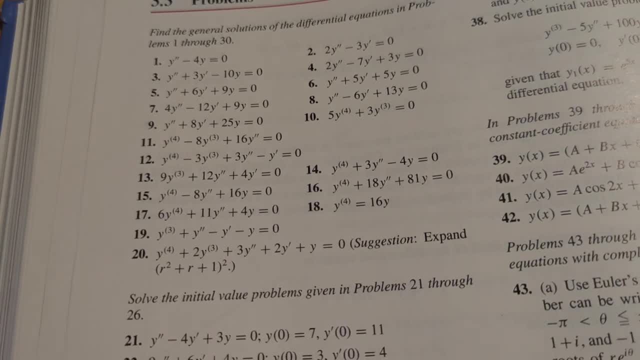 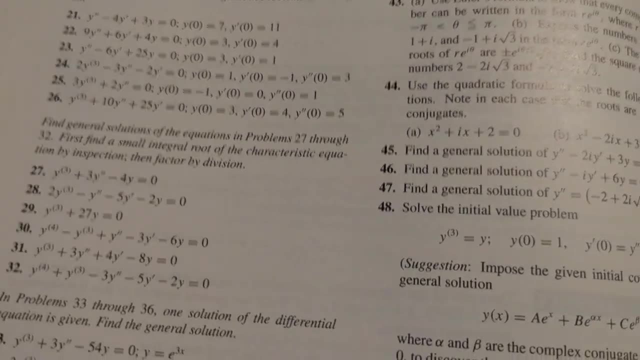 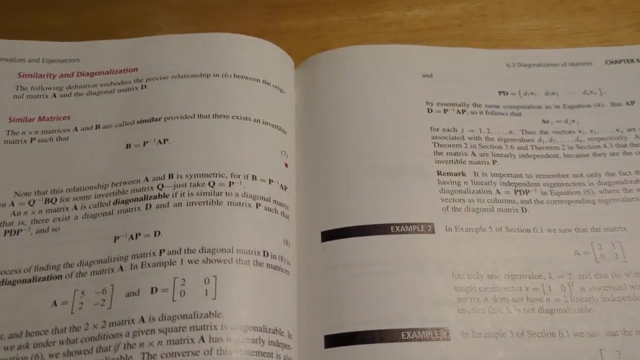 really easy problems. Some of them are a little bit harder, Some of the higher ordered ones. Then here you have some initial value problems- Again not hard, Just pretty easy stuff actually. Yeah, a lot of differential equations isn't too bad, But that's true of most mathematics, once you know how to do it. And here we. 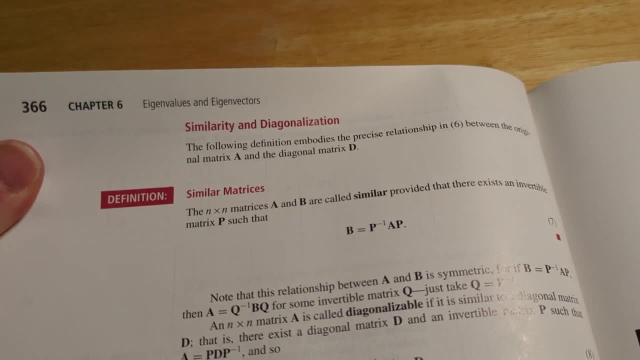 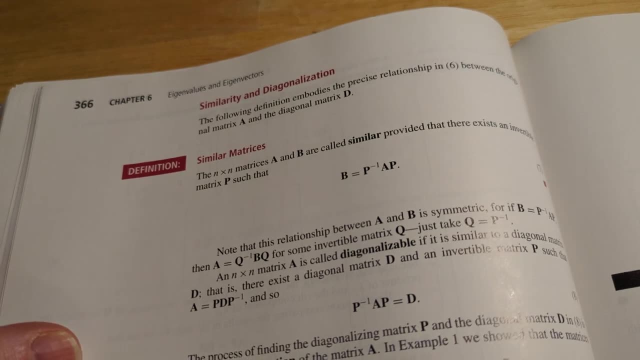 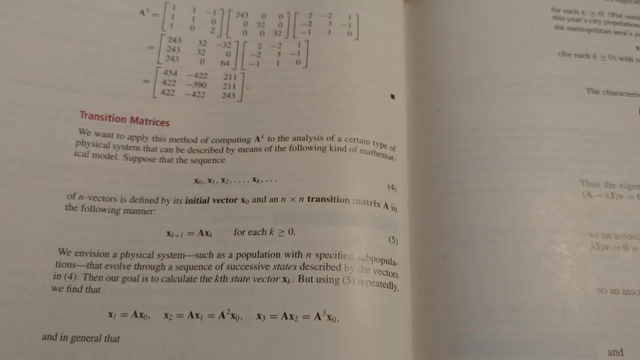 have some of the linear algebra, Similarity and diagonalization. So this is in a linear algebra textbook, Okay, but it's in this book as well, So makes it pretty cool. Yeah, I learned this in linear algebra. So yeah, overall I think. 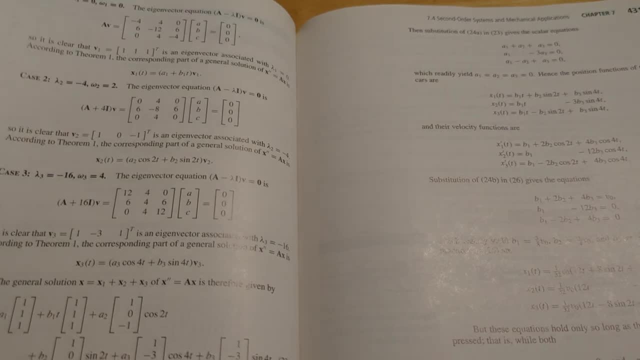 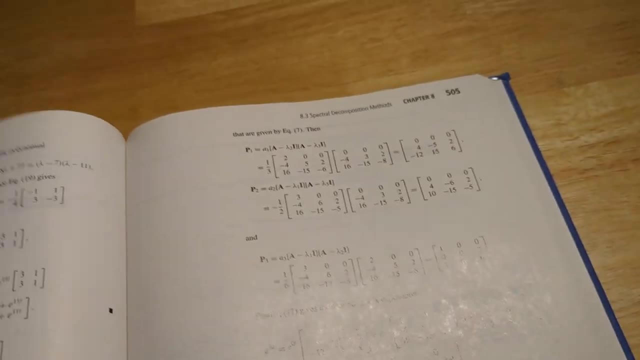 it's an interesting book, Very different from my other differential equations books, So I wanted to just talk about that and show you that it does have a lot of linear algebra in it And I think it's pretty good. It's pretty good, Let's. 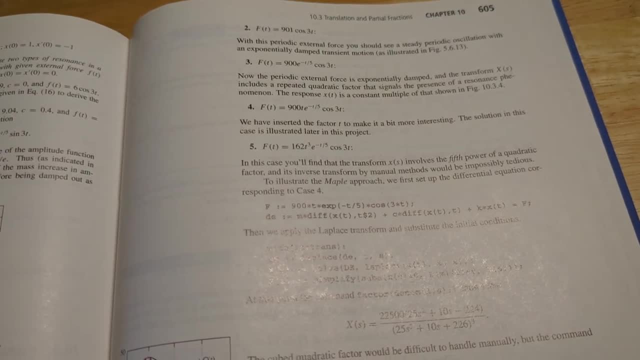 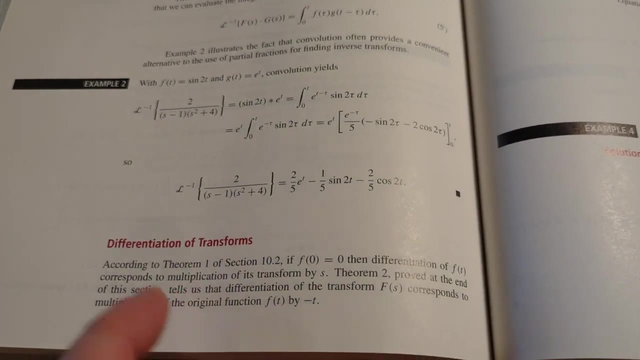 go to the Laplace transform section. Let me see, I think it's here. Yeah, this is the Laplace transform section. For example, it talks about differentiation of transforms. You'll find that in most books. So that's something that you find in most books: An integration of 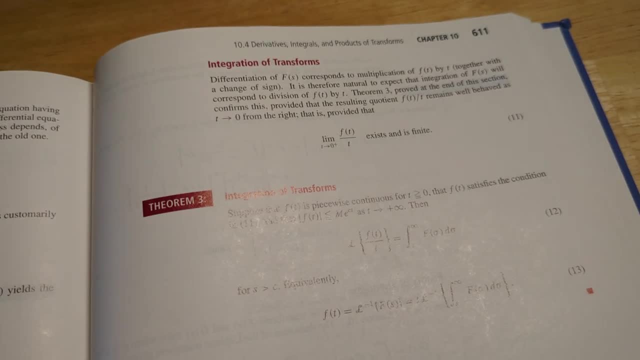 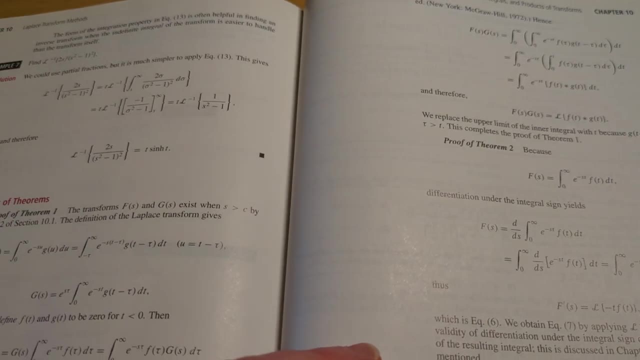 transforms. That's not something you find in every book. A lot of books do have it, But not every book has it. So kind of an interesting topic there. Then you've got the proofs of some theorems. Then you have there's the unit step. 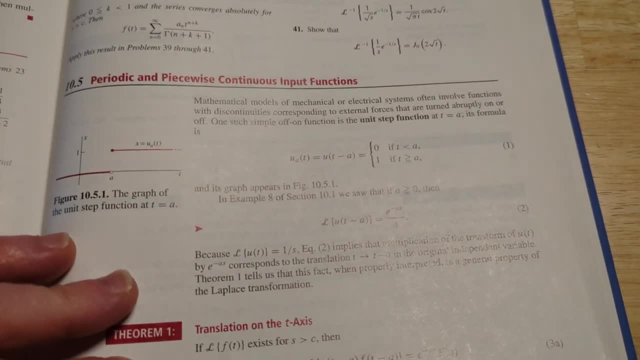 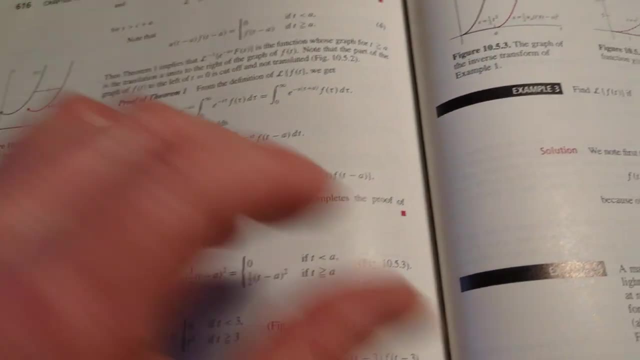 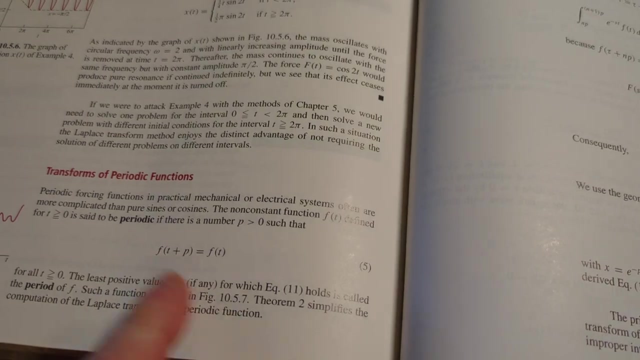 function That can be defined different ways depending on the text you're using. We have some more mathematics here. Yeah, it's just a nice textbook. Pages are really nice, Feels like it's good quality. Transforms of periodic functions: If you go into like electrical engineering, So like if you think that's. 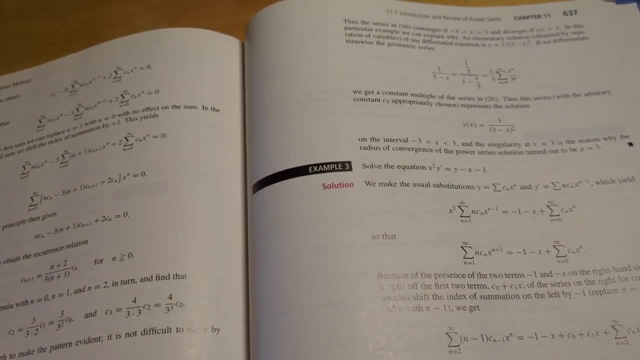 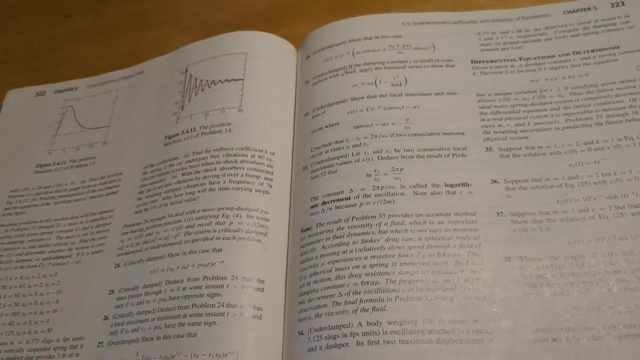 gonna be your major. This is a great book for that because this has a lot. I feel like it has a lot of content that can help you, Especially the Laplace transform stuff. They do a great deal a good job. but yeah, i like the book. i'll try to leave a link in the description and, if you found 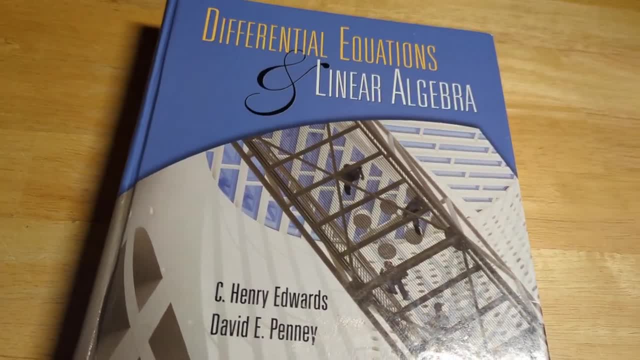 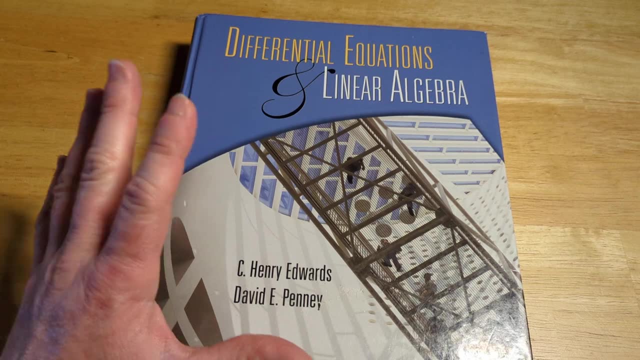 any value in this content. feel free to hit subscribe if you want to. oh also, before i forget, if you want to learn math, i do have math courses. they're on my website, math sorcerercom, so please use the links there. uh, they're actually on the udemy platform, but on my website i've got the 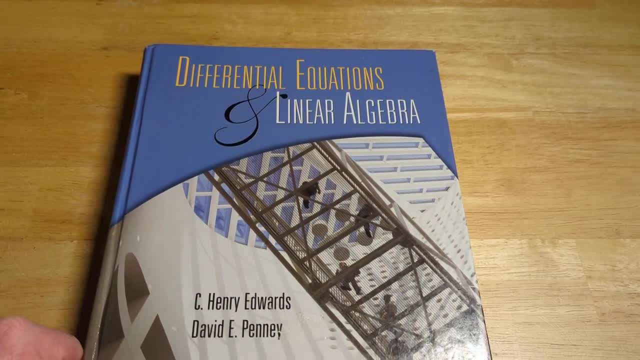 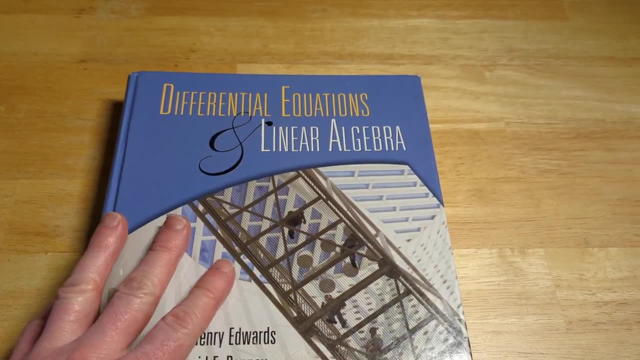 links and when you use my links you get a low price, because i actually lowered the price to the bare minimum so that you should get a low price always if you use the links from my website. i've got a couple courses on differential equations. they're both good. uh, some courses. 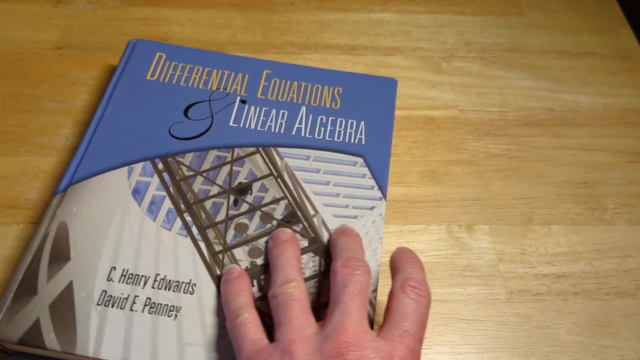 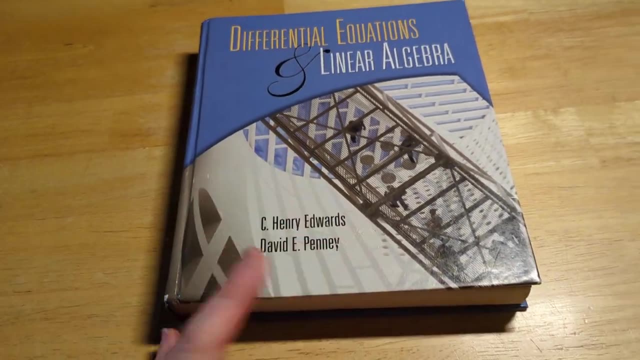 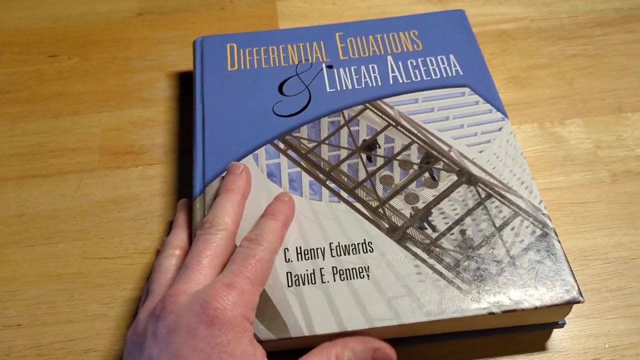 on calculus, advanced calculus, abstract, algebra, etc. yeah, i gotta give it a whiff here, just ah, it's nice. what a great book. yeah, very unique because it has linear algebra and again, i feel like a lot of the topics like little subtopics in the sections you won't find in. 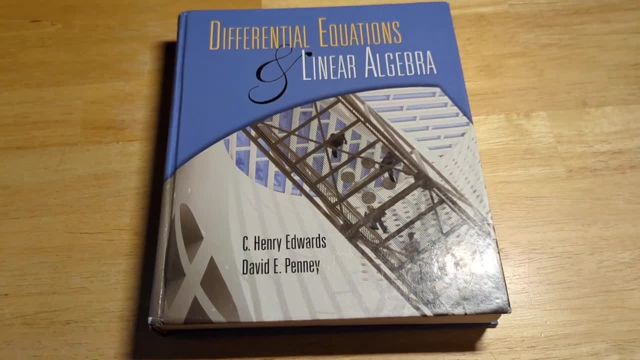 other books, very, very different other books, and i do like it. i hope it's been helpful. keep doing math.